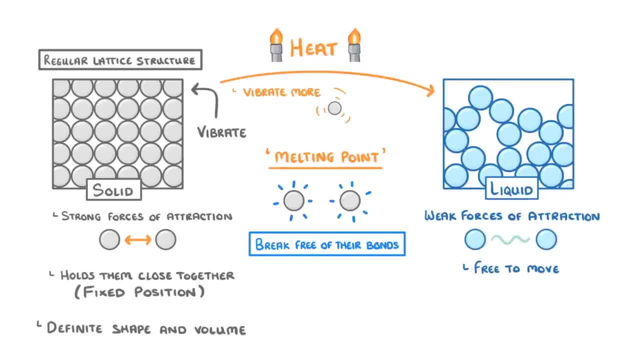 particles, So they're free to move around and are arranged pretty randomly. However, the weak forces of attraction do mean that the particles tend to stick together and are fairly compact. This means that they have a definite volume, even though their overall shape can change, allowing them to flow to fit a particular container. 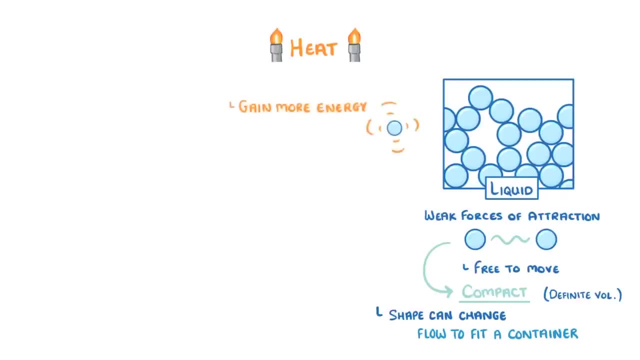 If we then heat up our liquid, the particles will again gain more energy and this will make the particles move around faster. This weakens the forces holding the particles together. Then, once we reach the boiling point, the particles will have enough energy to break. 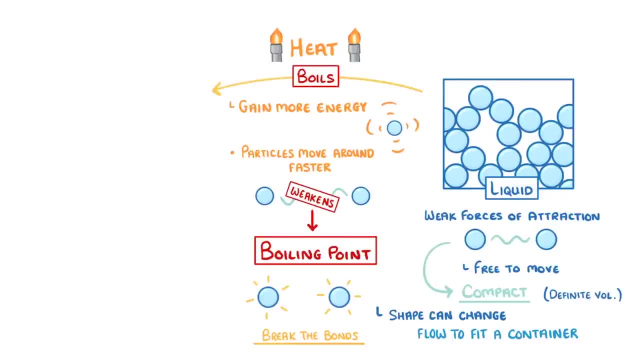 the bonds altogether, and so the liquid boils or evaporates into a gas. In gases, the force of attraction between the different particles is very weak, so they're basically free to move around by themselves. This means that gases don't keep a definite shape or 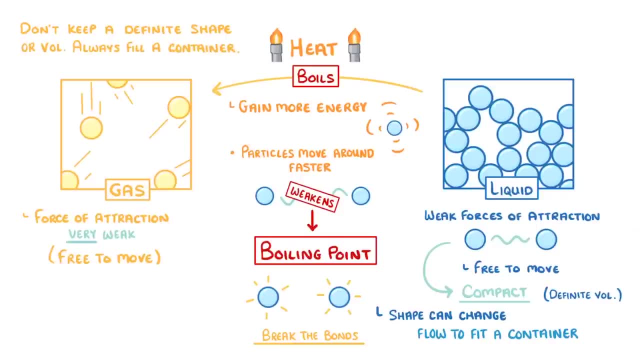 volume and instead will always fill a container as they spread out as much as possible. Now we normally say that gases are constantly moving, with random motion, which is a bit confusing, because gas particles actually move in straight lines, They don't randomly swerve. 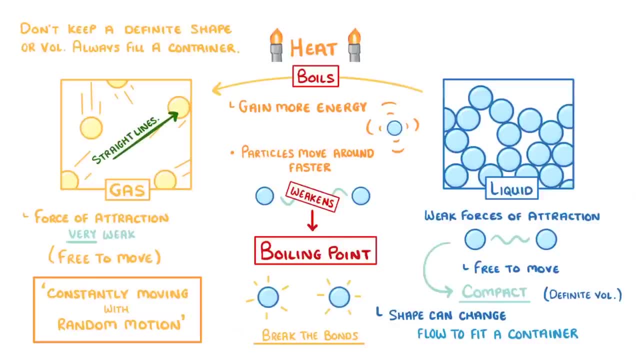 What we really mean by random motion is that the particles can travel in any direction and they'll end up being deflected by solid walls and other gas particles. These are called non-s丈 gas particles. They can move in any direction or they'll. 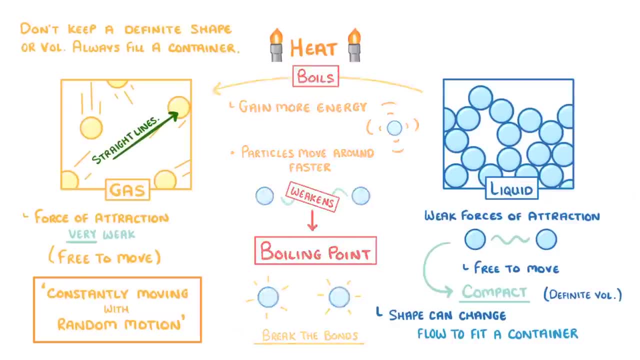 walls and other gas particles randomly. When we heat up a gas and the particles get more energy and so travel faster, the gas will either expand if the container it's in is expandable like a balloon, or if the container is fixed. then the pressure will just increase. 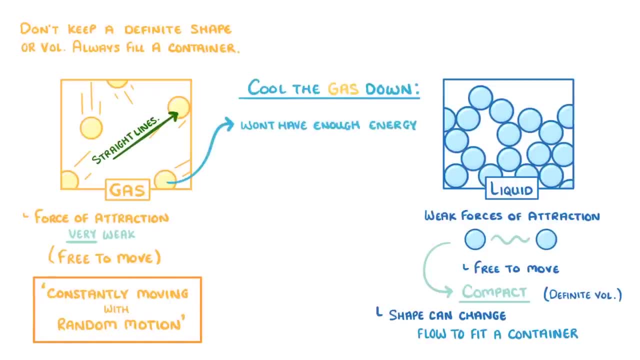 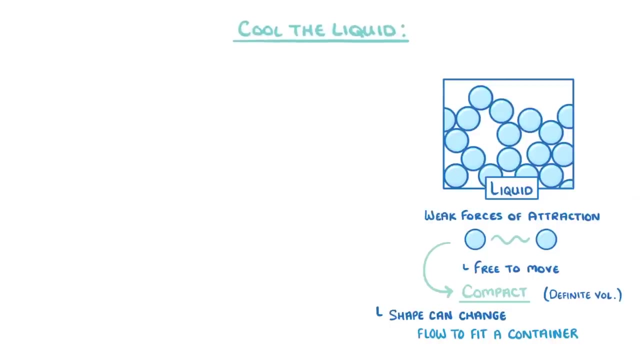 On the other hand, if we cool the gas down enough, then the particles won't have enough energy to overcome those forces of attraction between them, and so bonds will start to form between the particles, condensing the gas into a liquid. As we cool down the liquid even further, the same thing happens: The particles won't.